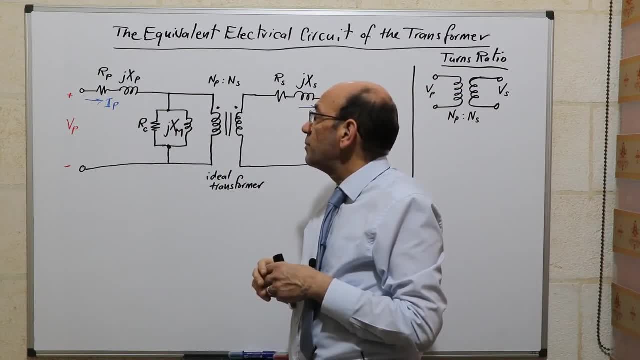 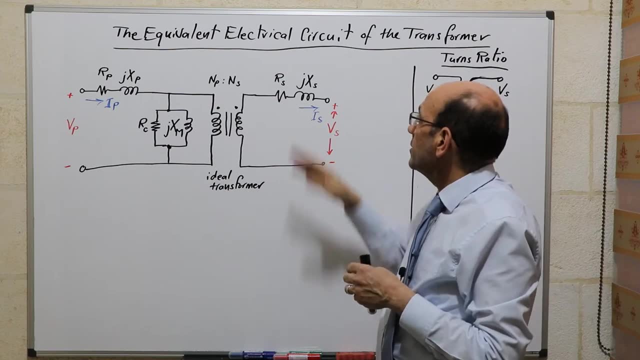 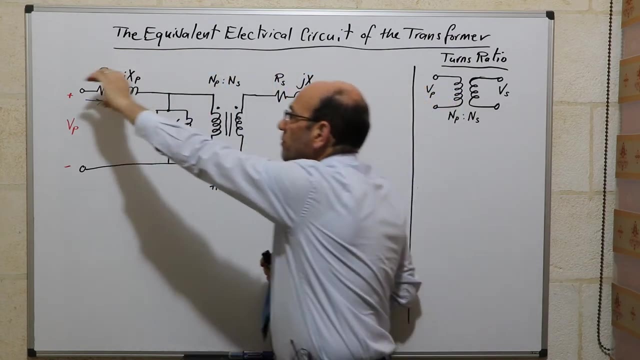 of the secondary And we've referred that or denoted it as XP And the same for the secondary. So any leakage flux is represented as X subscript S for secondary. Then we actually we have allowed for the shunt components. So these were the series components We've also allowed. 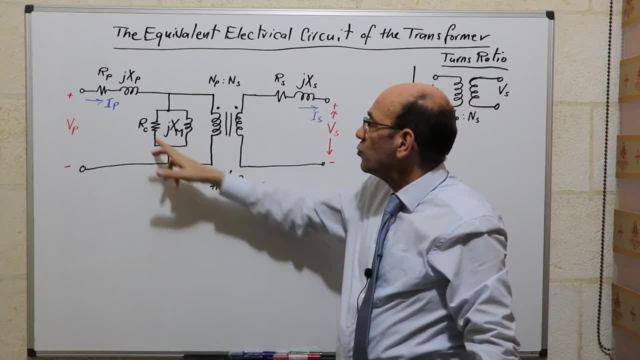 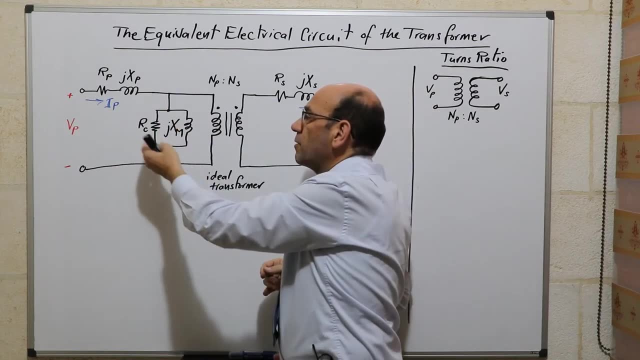 for the shunt components. And the shunt components are made of two components which are connected in parallel: R, subscript capital C, which is the core losses. So these would represent the eddy current losses and the hysteresis losses, So they will account for these losses. 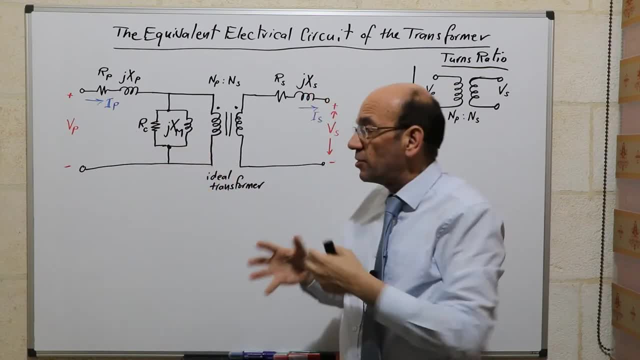 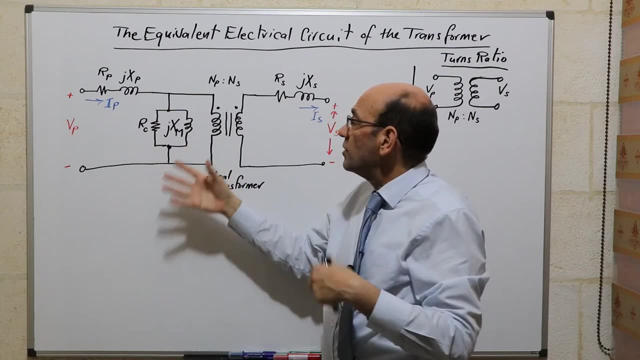 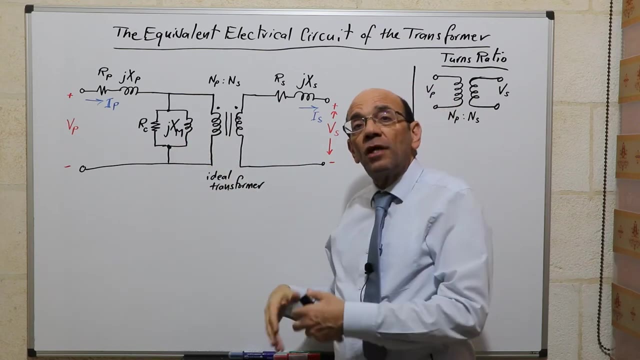 As I've said previously, there is no such thing as a resistor. It's not actually a physical resistor that we can find or see. It's actually a means of representing these core losses by using a resistor. The other component which actually we've accounted for is the fact that we have what is called 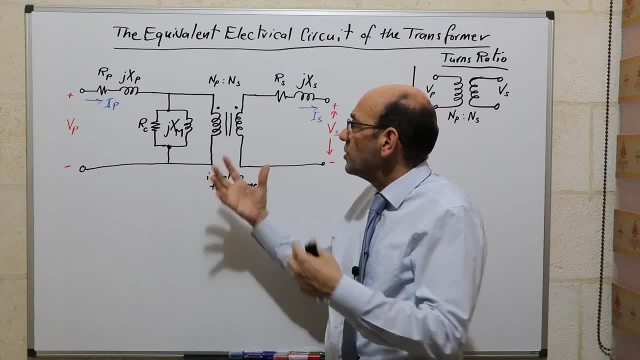 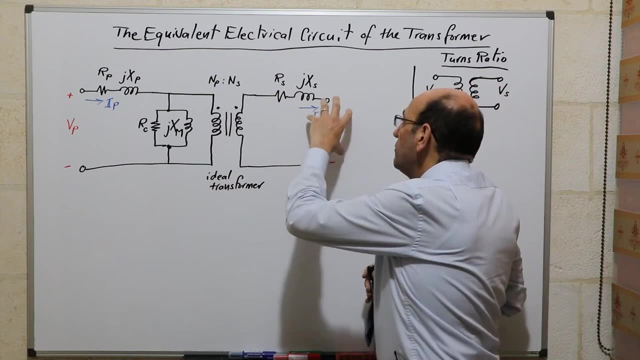 a magnetization current And that magnetization current actually magnetizes the core and actually exists, even when there's no load on the secondary. So you would see, here, even when there's no load is connected, here- and this is open circuit- there's still some magnetizing current. 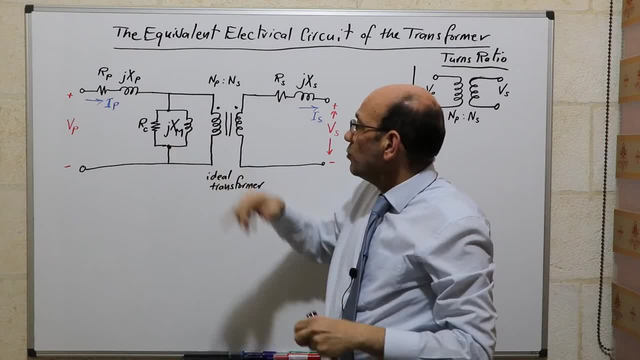 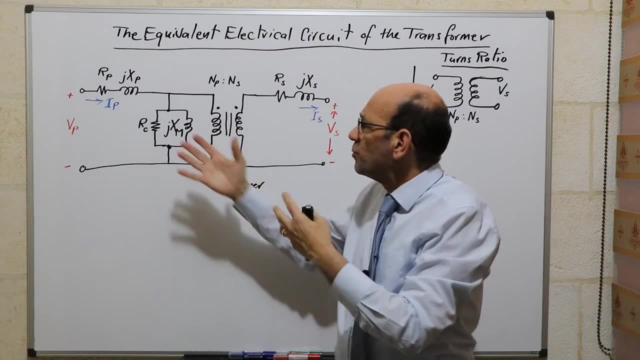 So this is the magnetization current flowing in the transformer And this component, which is an inductor, accounts or represents this magnetizing current. And the magnetizing current was observed to lag the voltage by 90 degrees. And the best component to represent a current. 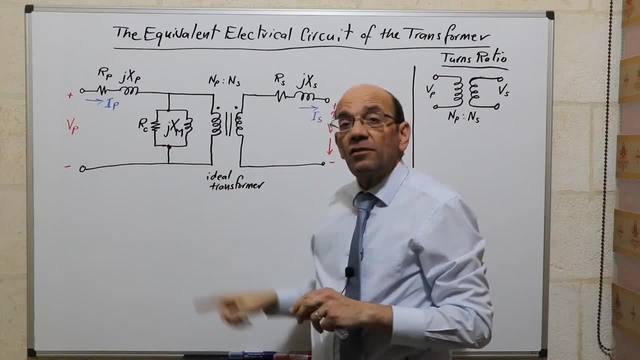 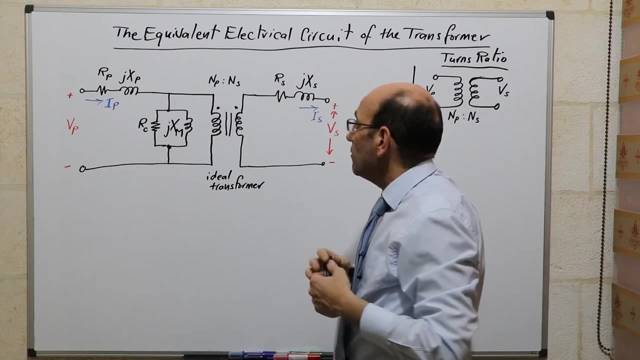 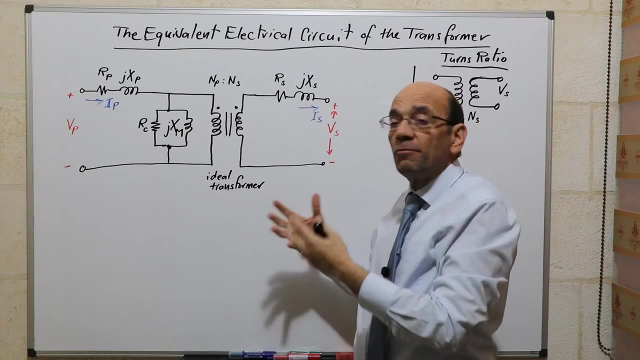 lag of 90 degrees with respect to the voltage is an inductor, And so this actually completes the equivalent electrical circuit model for a single phase transformer. What we'd like to do today Is to start simplifying this model to make it much more practical to use in real life. 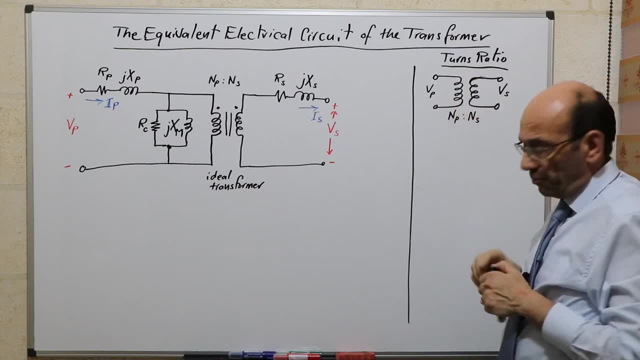 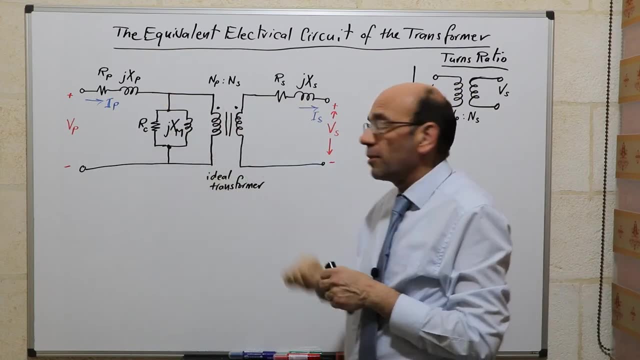 And to do this we actually go to the turns ratio, Because the ratio we want to use this to actually be able to reflect the secondary into the primary. We want to see what does the secondary part look like when we see it from the primary, And to do that we actually 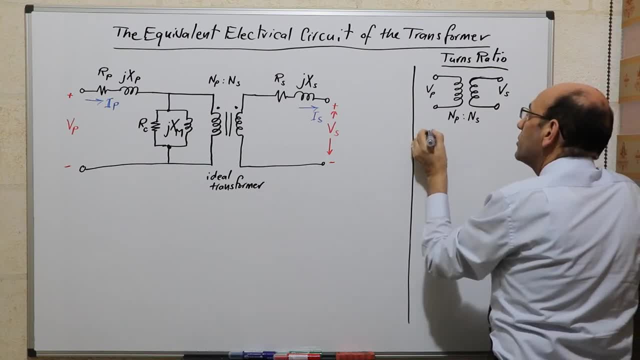 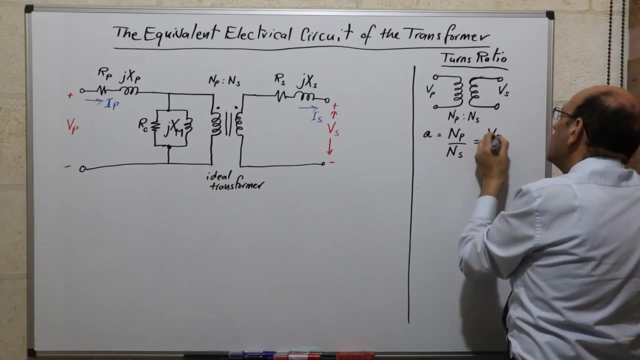 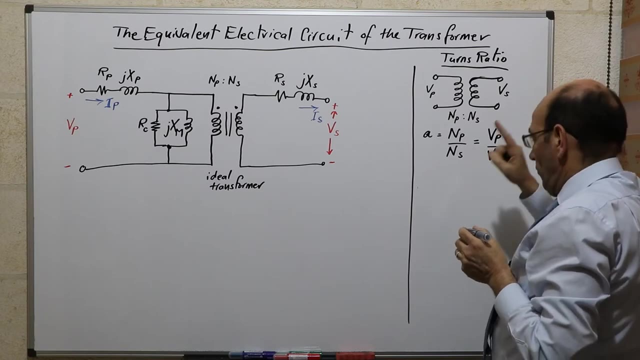 resort to what is called the turns ratio, And the turns ratio is actually the ratio between the turns of the primary to the turns of the secondary, which also is actually the voltage of the primary with respect to the voltage of the secondary. So, for example, if A is 10, this means this is a step-down transformer. because when we say 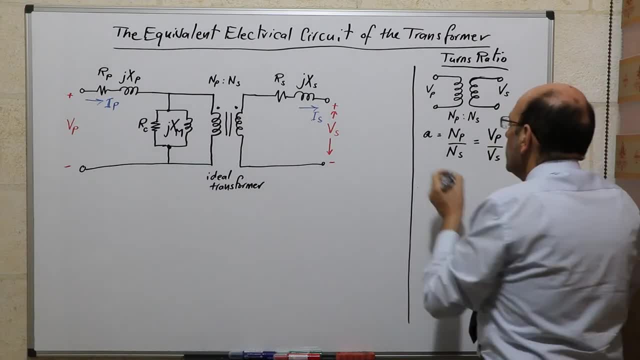 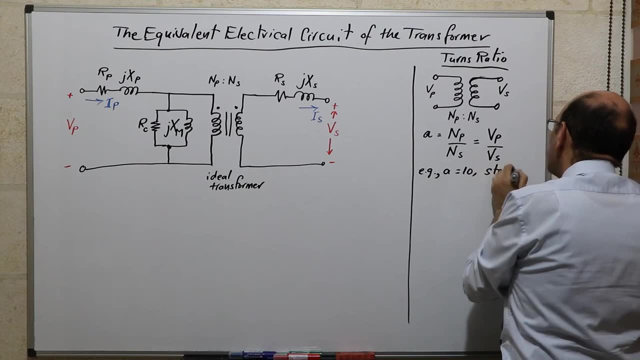 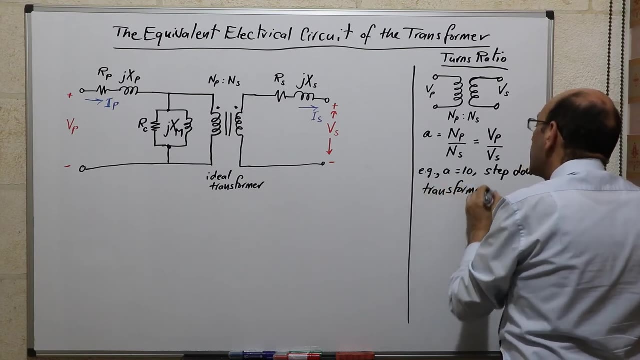 step-down we're referring to voltage, not current. So, for example, if A is equal to 10, then this is a step-down transformer. Do a great job. Thanks down transformer, which means it is stepping down the voltage. so when we use the term step down, 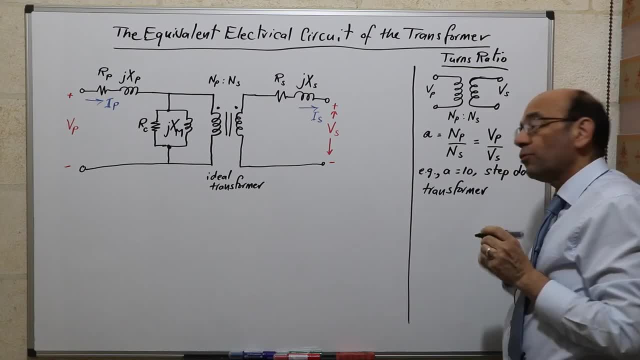 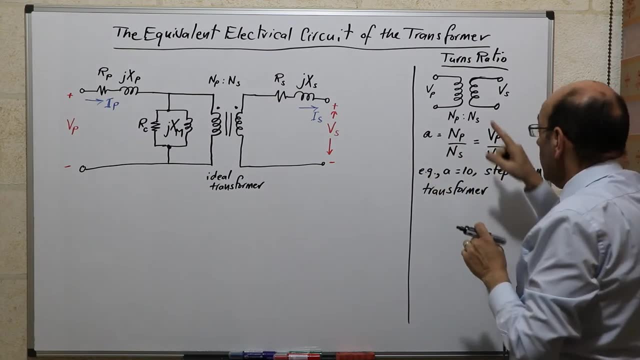 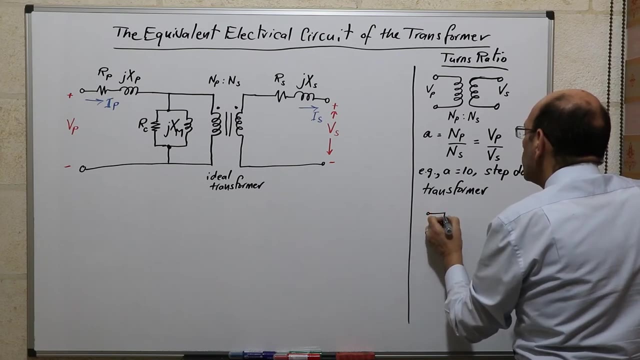 we're talking about voltage. when we use the term step up, we're also talking about the voltage, and the ratio of the number of turns is the same as the ratio of the voltages. so let us assume we wanted to try to represent this transformer in a with a load. so if this transformer had a load at 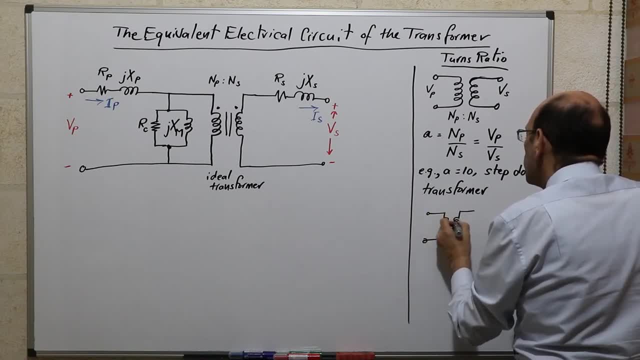 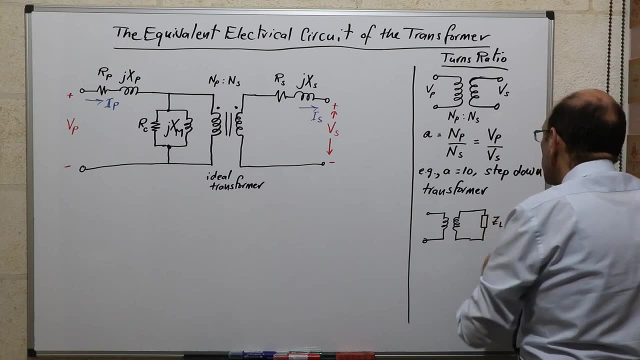 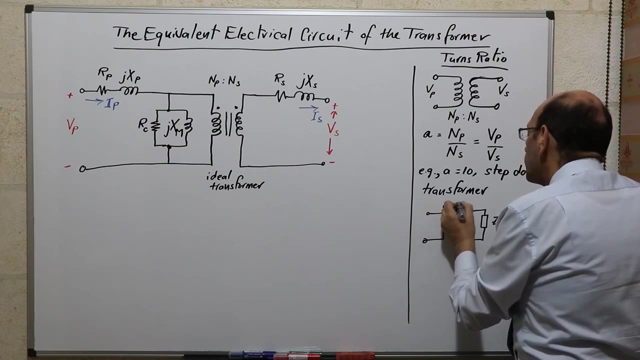 the secondary, connected to the secondary, and let's assume this was an impedance, and it was an impedance of, let's say, z subscript capital L, meaning it's a load, the impedance of a load, and here we have a to one, which is the turns ratio, and we're asking the question: what would this? 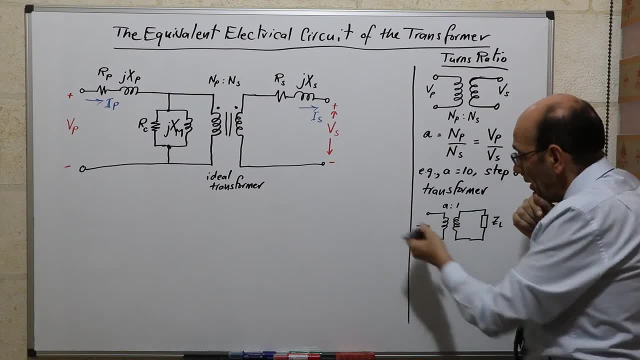 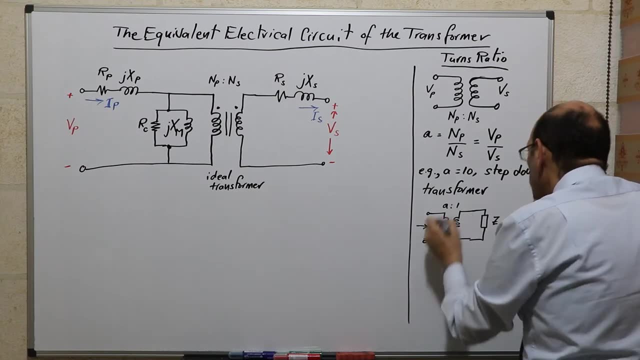 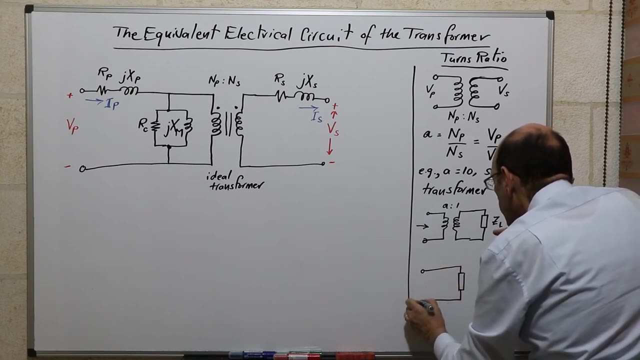 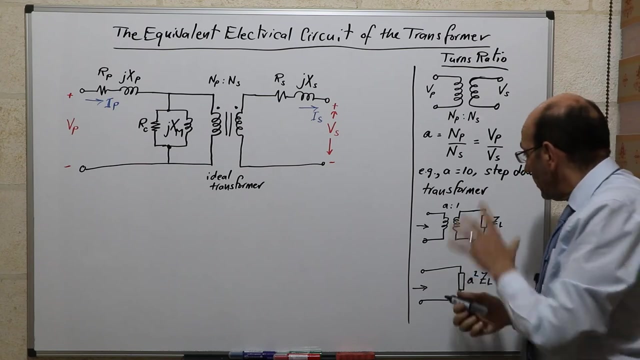 what would this impedance look like if we actually want to see it from the primary point of view, and we can prove that actually this circuit can be simplified as follows: so we can actually have a square z L and in fact this circuit will be equivalent to this circuit from the point of. 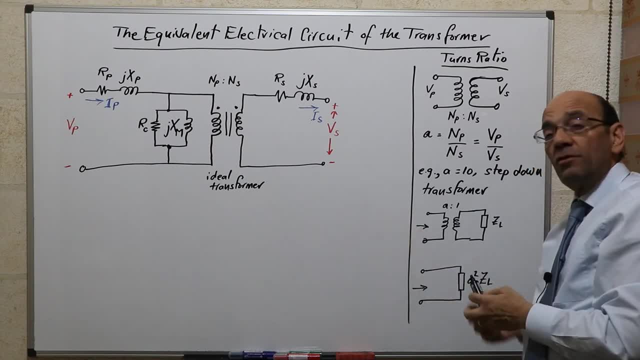 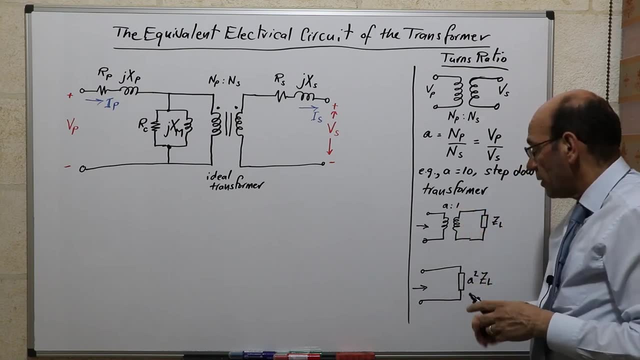 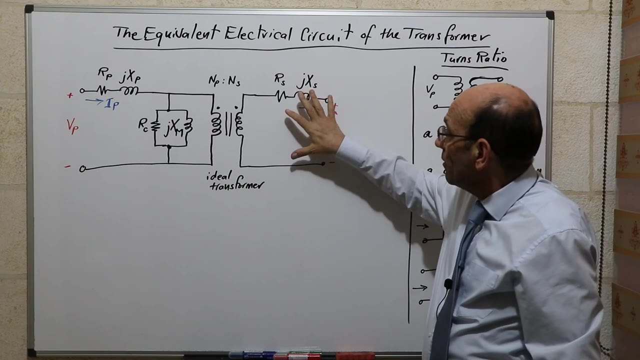 view when we see it from the primary. so, when looking through this point, we actually see z L multiplied by a square, not by a, by a square, and we will use this now. we will use this representation, this simplification, to try to reflect this onto the primary.